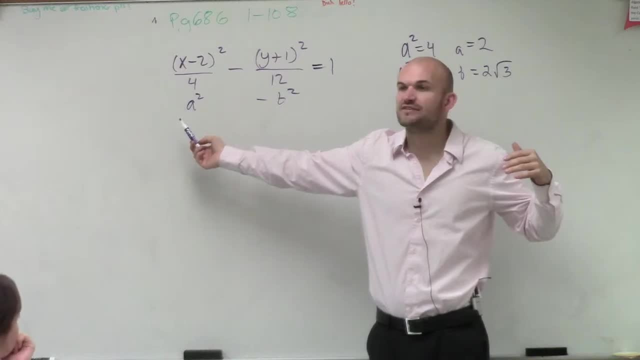 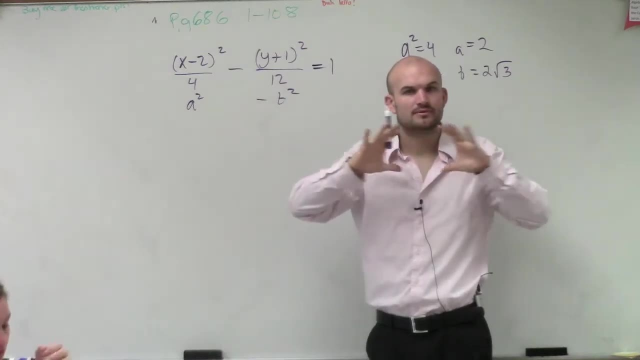 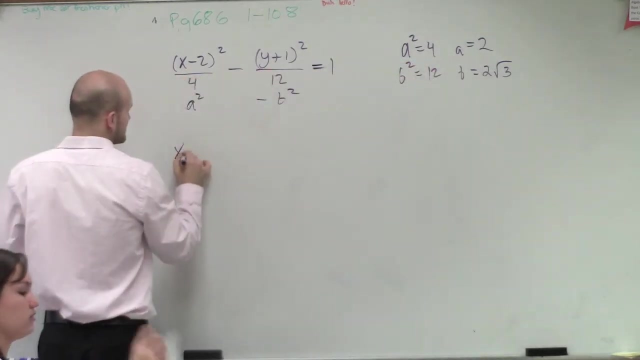 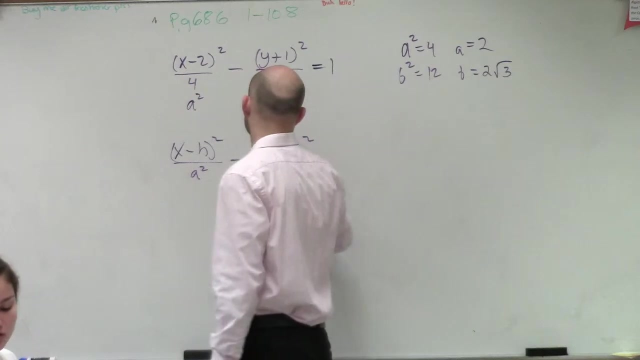 If my x squared is my coordinate over my a, does that tell me if it's vertical or horizontal? What is my transverse axis going to be? What are my openings going to be? Horizontal or vertical? Horizontal, Horizontal? Why? Because it's always So, if you guys remember here's. 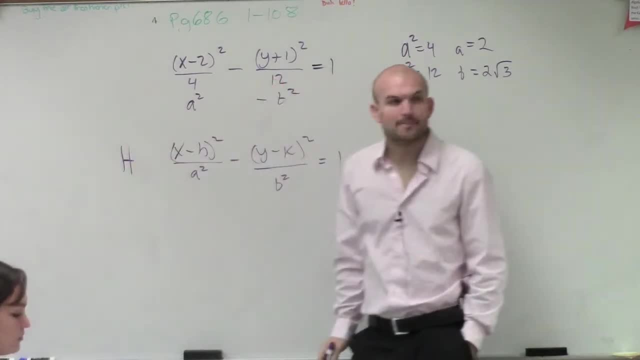 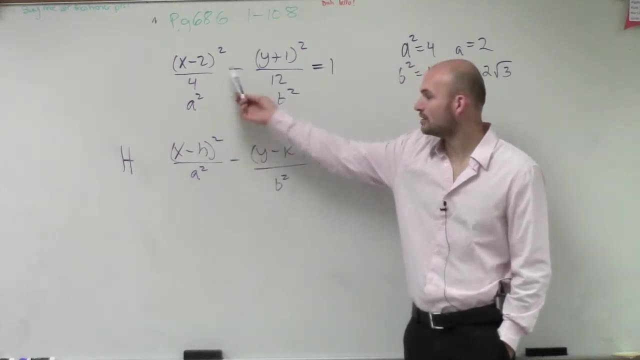 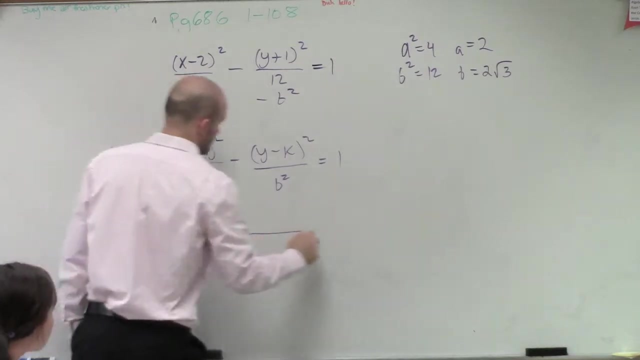 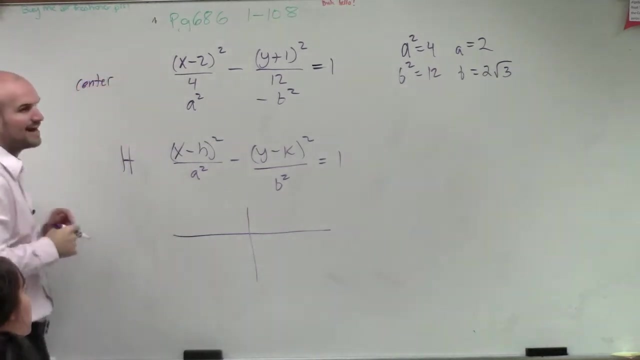 our equation. for our x squared, There is no frotional lambda lasting watching for external time. What's important about that is I know that now, if I find my center And I'm just going to sketch this, You don't have to sketch this to all this work, But I want to show you the. 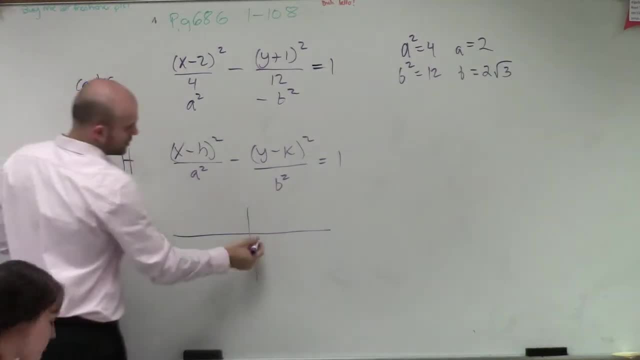 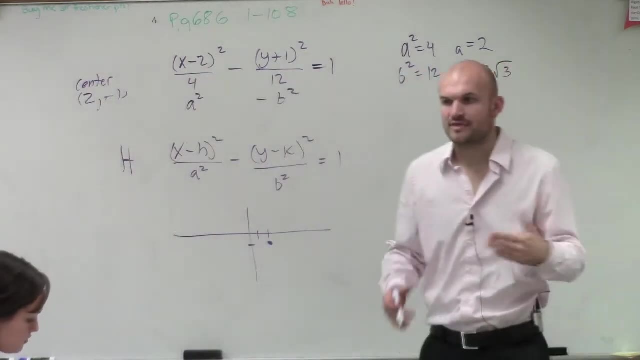 center is going to be 2 comma negative 1.. 2 squared 1, comma negative 1.. Now, since we said it's horizontal, that means my vertices and my foci are all going to lie on our horizontal line, which. 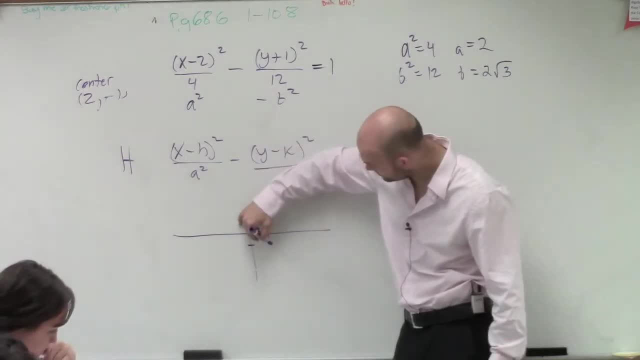 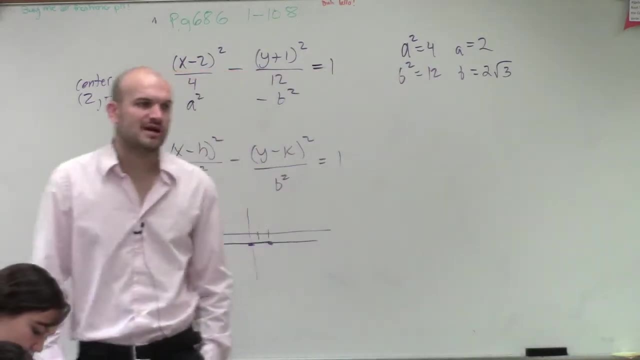 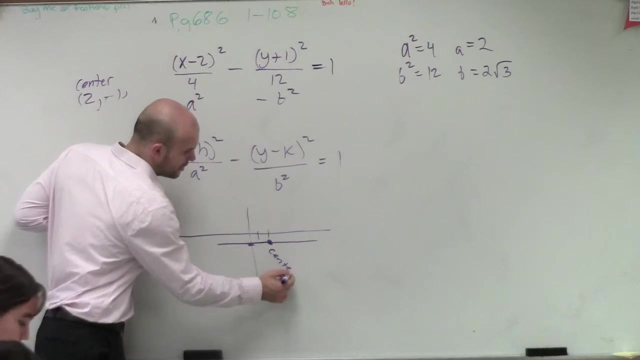 we call the transverse axis Very good. So now what we need to do on this transverse axis is find our foci and center. So, ladies and gentlemen, we know this is our center. We know that the foci, Ryan, and the vertices. 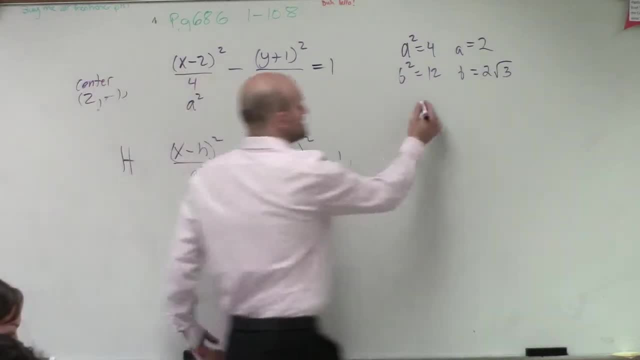 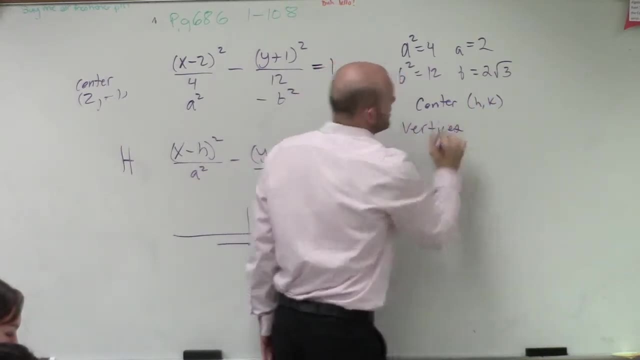 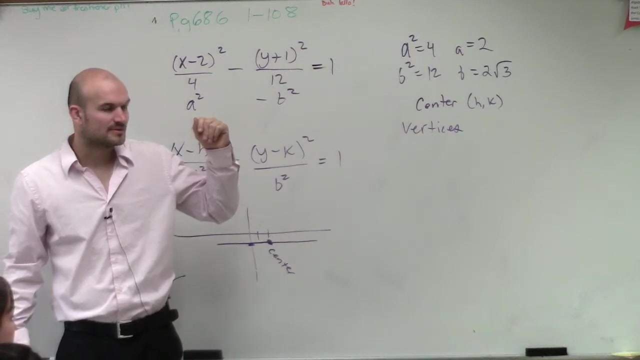 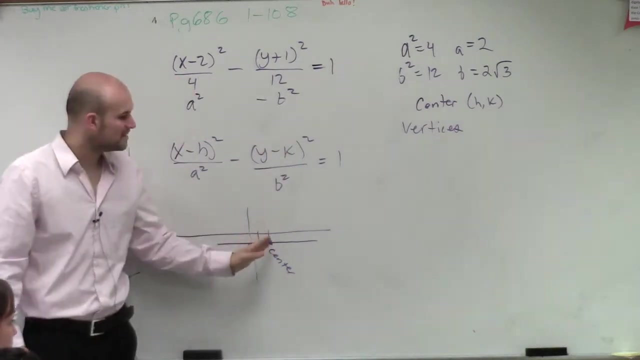 all lie on this line. So if we know the center is h, comma, k, the vertices- remember the vertices- is the distance of what from the center Hazel Vertices, to the alphabet First letter in the alphabet A, A: The distance from the center to your. 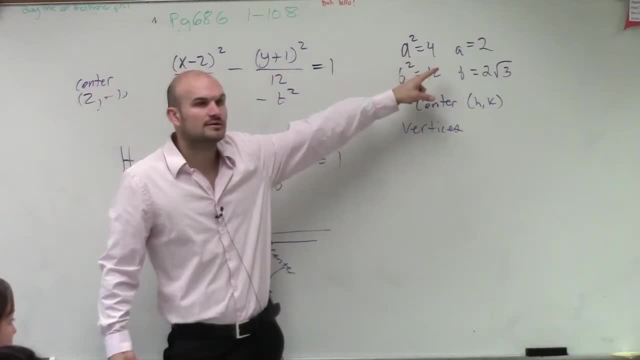 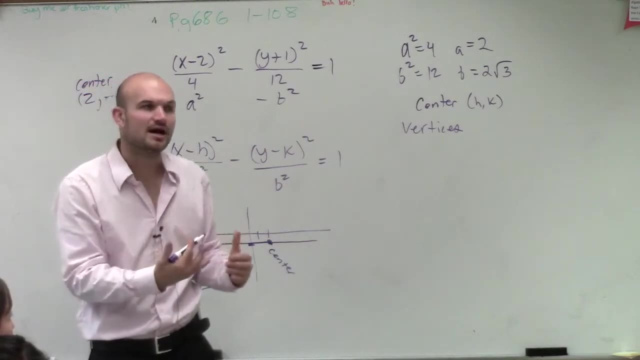 vertices A. The distance from the center to your vertices is your length a. So our length a is what 2. 2. So therefore, remember, we have our vertices to the right and to the left. Why is it to the right and left again? 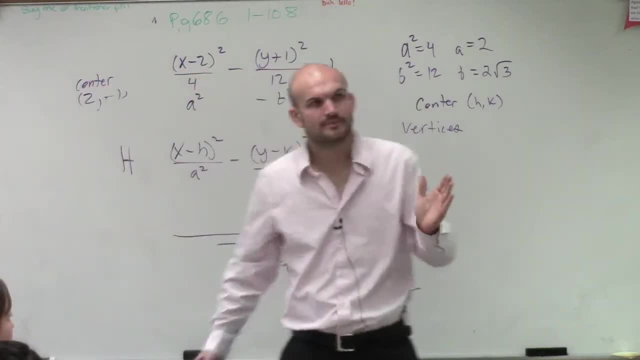 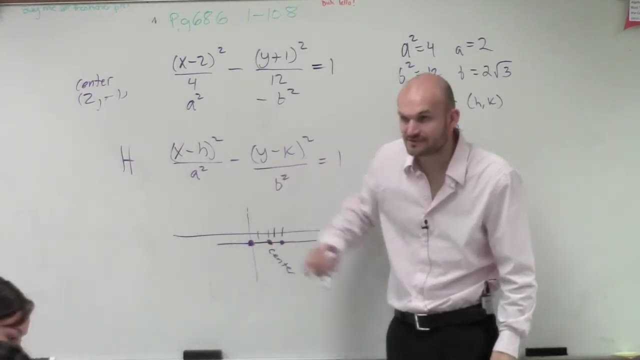 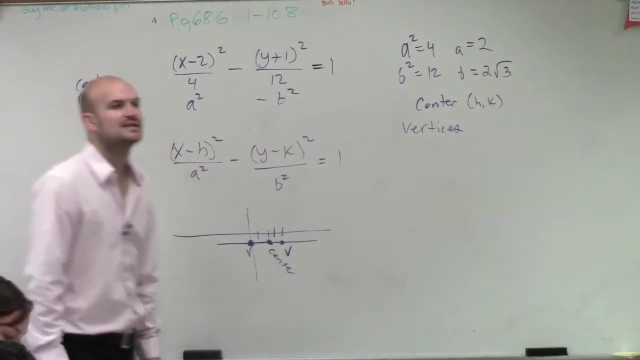 Because we determine from our equation that we have a horizontal hyperbola. So, therefore, I'm going to go over two more units to the right and I'm going to go two units to the left. Now, what I have just found out are my two vertices. 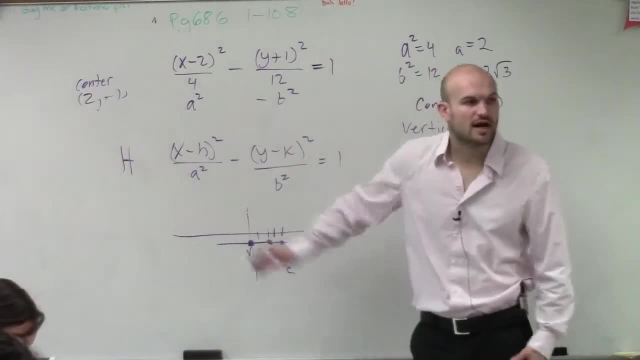 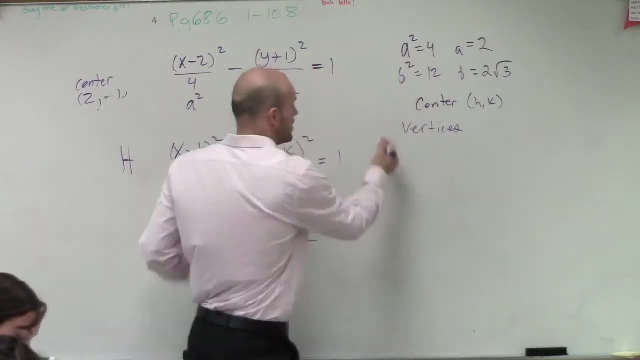 Does that make sense, Kirsten? Yeah, OK, So you've figured out your two vertices, all right. The other way to look at this, ladies and gentlemen, when you have vertices, that is horizontal, as long as it's horizontal. what did I really do? 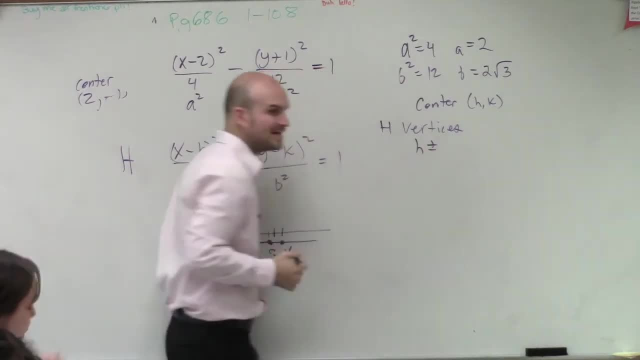 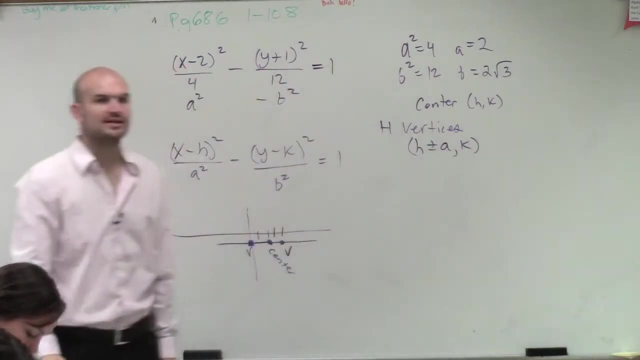 I took my center and what I did is I added and subtracted my distance a. So if you guys just wanted to algebraically do this without actually drawing the graph, all I simply did is I added and subtracted a to my h comma. 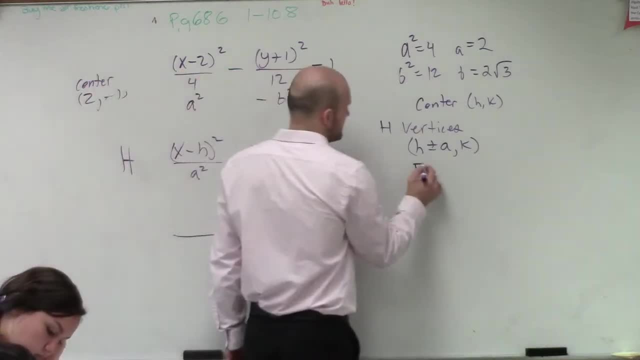 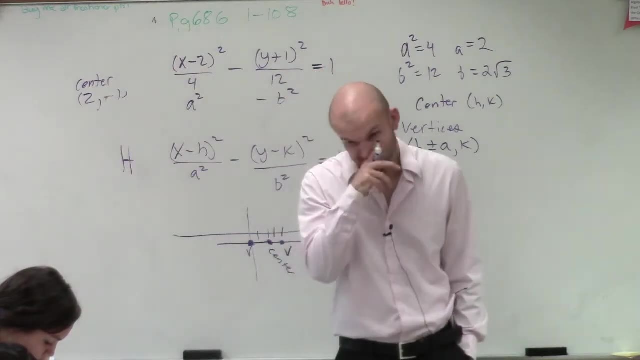 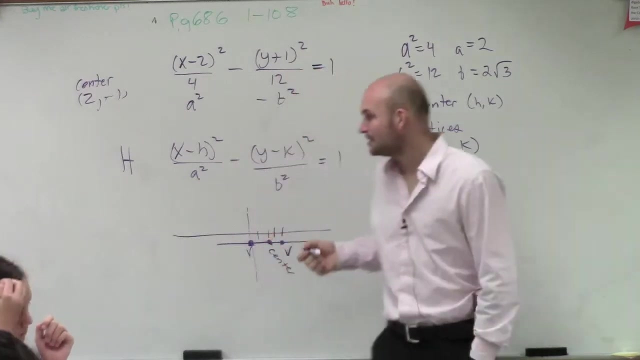 h-coordinate of my center. Now to find the foci. the distance of the foci is going to be what? from the center? Bjory, Exactly, It's the third letter in the alphabet c, right, And that's why we had you writing this down. 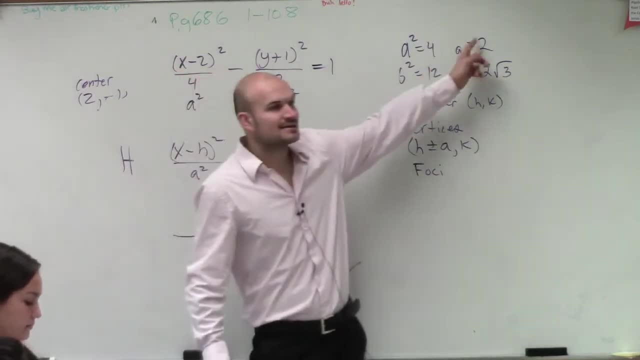 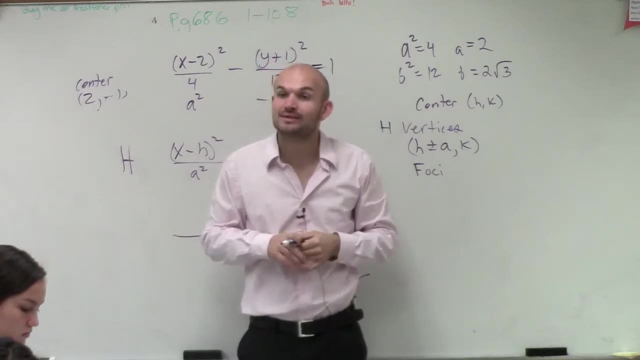 So we need to figure out what c is. I know what a is, I know what b is. I do not know what c is. Now there was an equation over there which I showed you how you can relate to all three of them. 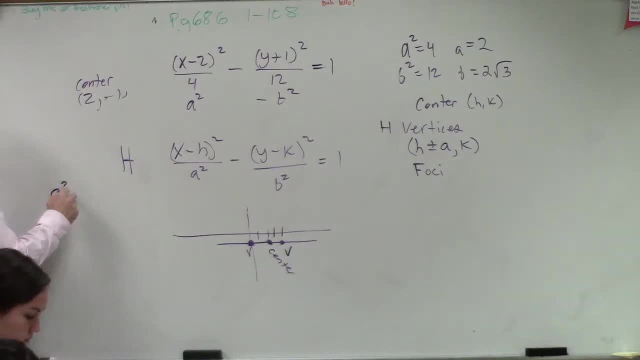 So our equation goes: c squared equals a squared plus b squared. So a squared is 4 plus b squared, which is 12, equals c squared. So c squared equals 16.. c equals 4.. So remember, as I spoke about this, 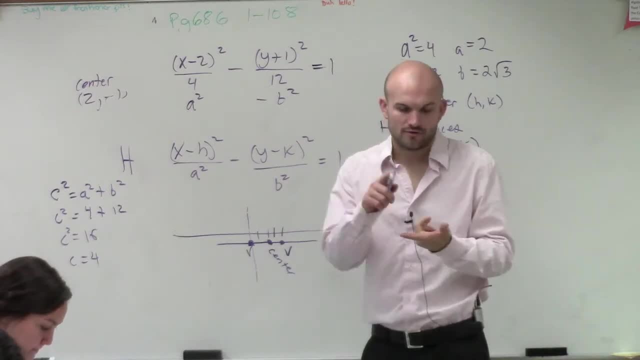 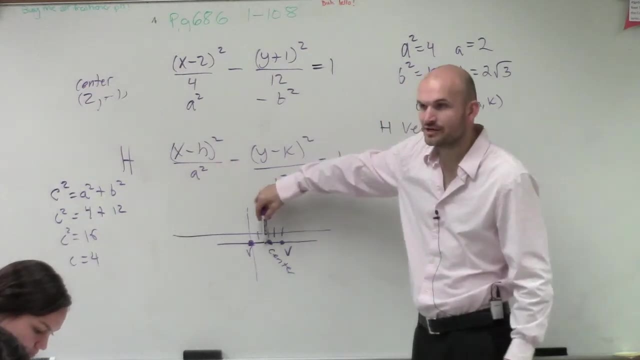 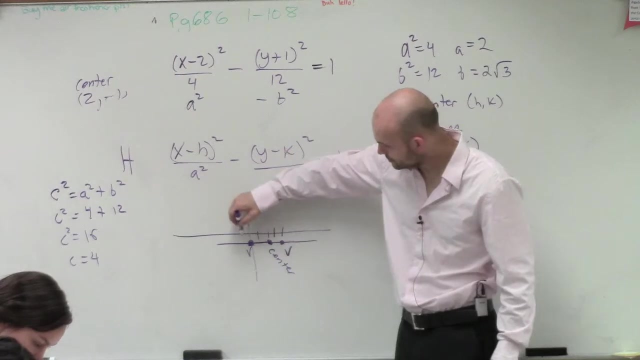 for a horizontal hyperbola. your foci and vertices and center all lie on the same axis. So if here's my center now, the distance to my two foci's is now 4.. So I need to go 4 to the left: 1,, 2,, 3,, 4.. 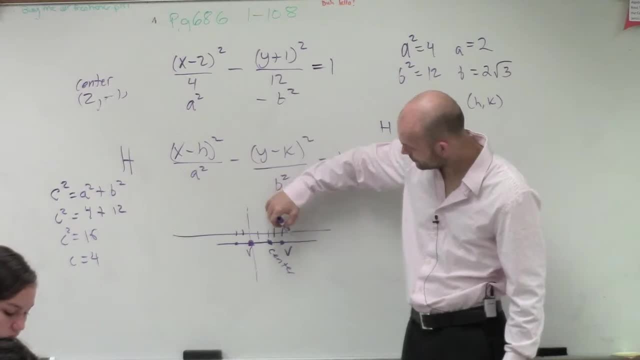 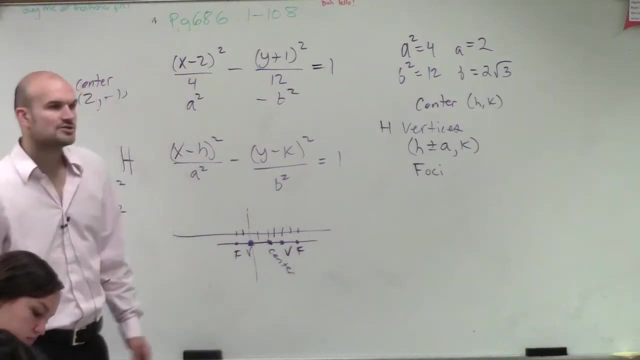 And I need to go 4 to the right: 1, 2,, 3, 4.. So now I've just determined what my two foci are. So what you can also understand is I'm really doing the same thing again. 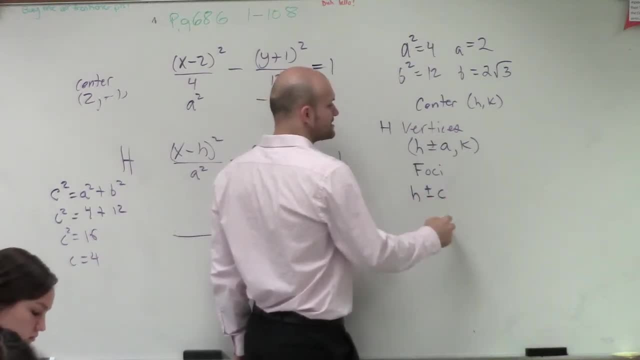 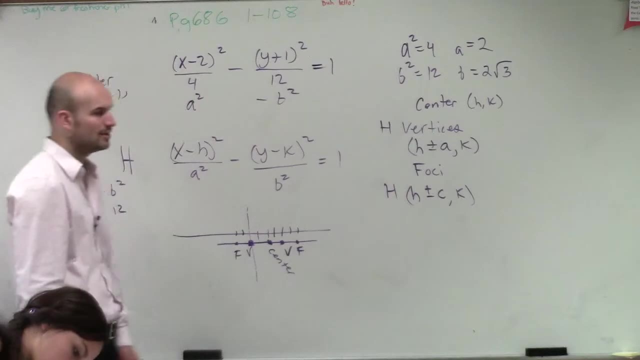 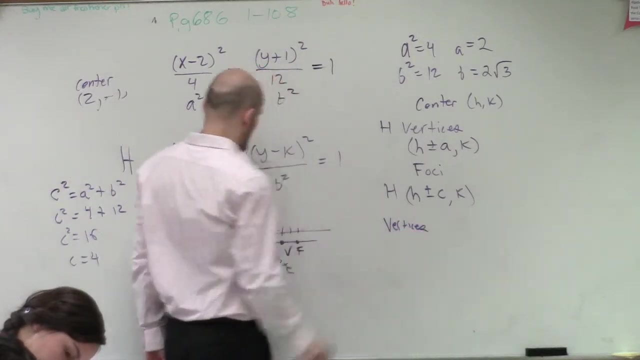 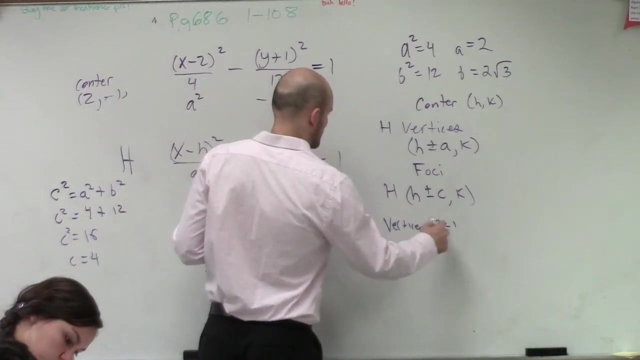 I'm taking my h and I'm adding and subtracting c from my h and my k. That's how we find the foci for a horizontal hyperbola. So now I just need to determine these points. So my vertices are going to be the points at 0, negative 1,.